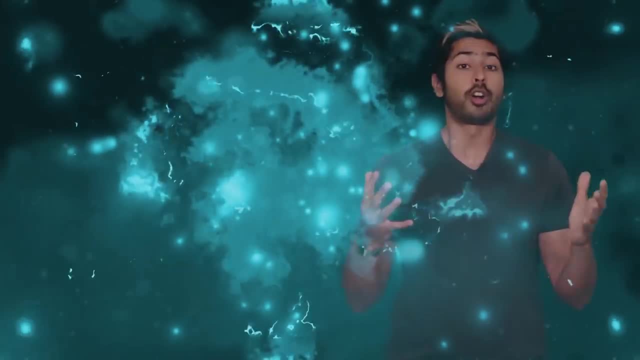 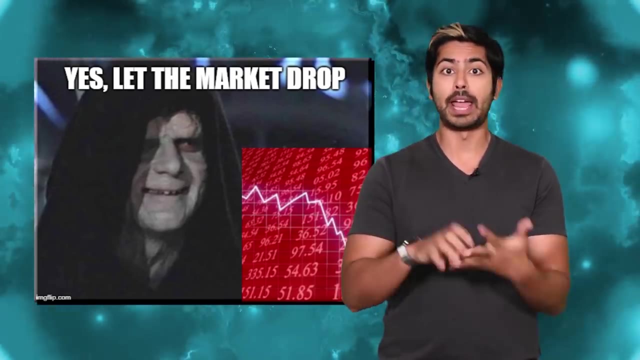 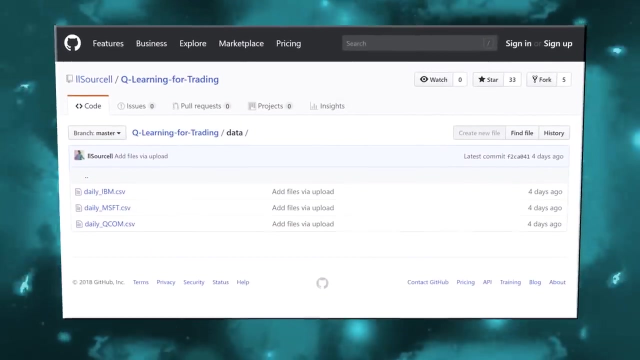 You can then tune your algorithm with sliders without using code. There are so many data points we could use that affect prices at different scales. News and rumors affect prices, micro and macro economic cycles, new laws. But let's start simple. Our starting dataset will be three CSV files. Each contains stock prices for 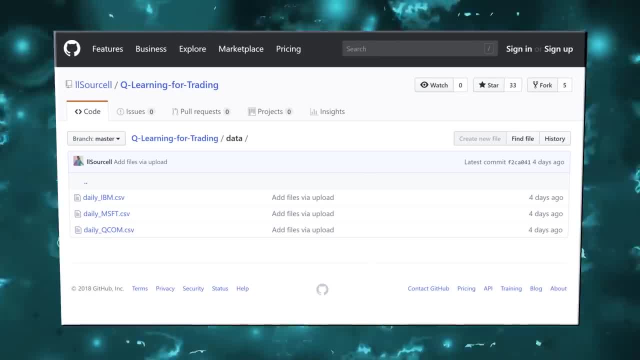 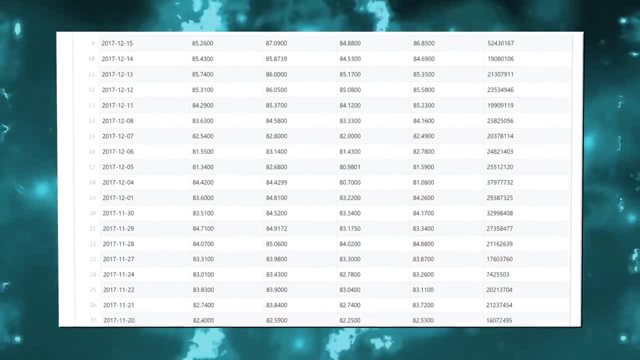 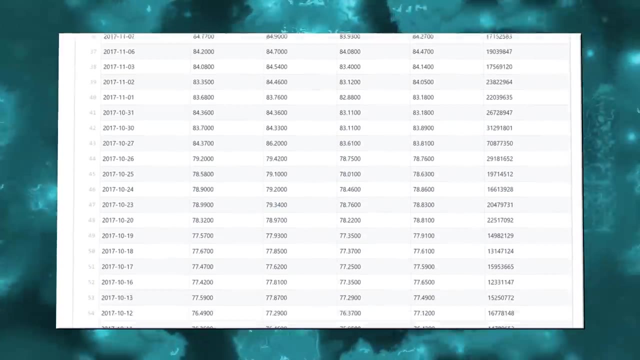 the past 17 years for IBM, Microsoft and Qualcomm respectively. The dataset was created using the Alpha Vantage API that lets us access both real-time and historical stock data. We'll want to build an algorithm that can learn from this dataset. Let's think about how to frame this problem. 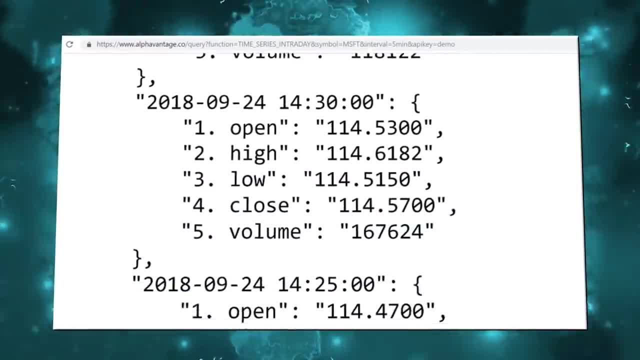 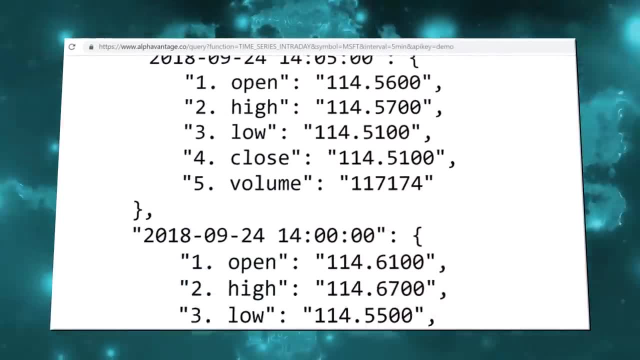 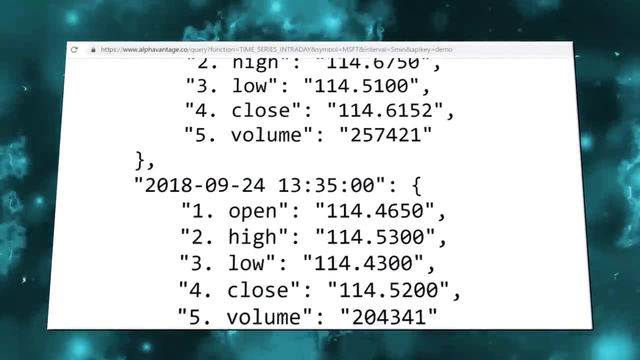 We have both historical data and access to real-time data via the API that can constantly pipe in updated prices, which we can add to our CSV files. This is a real-time environment where time is a dimension. We know, then, to use reinforcement learning, as it takes time into consideration. 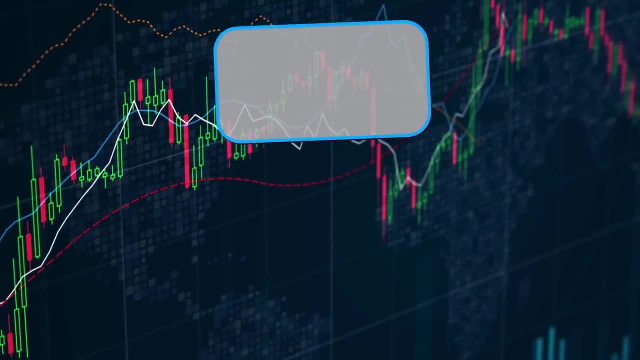 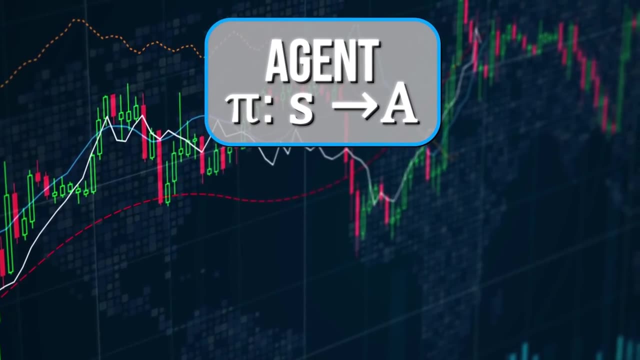 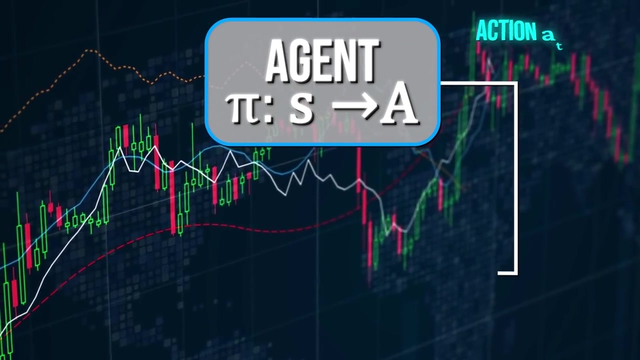 Using reinforcement learning. we can frame our problem as a Markov decision process, which consists of states, actions and rewards. Our agent will be able to execute an action in this environment and, luckily for us, the action space in this case is pretty simple. 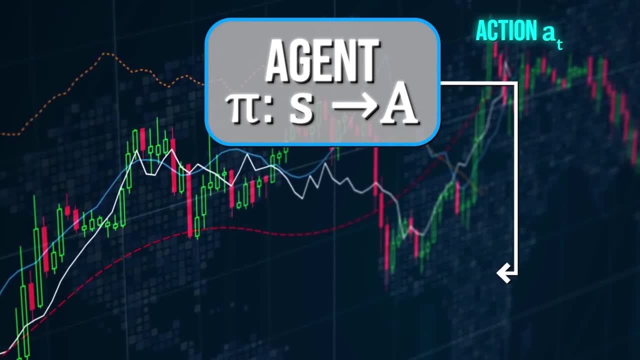 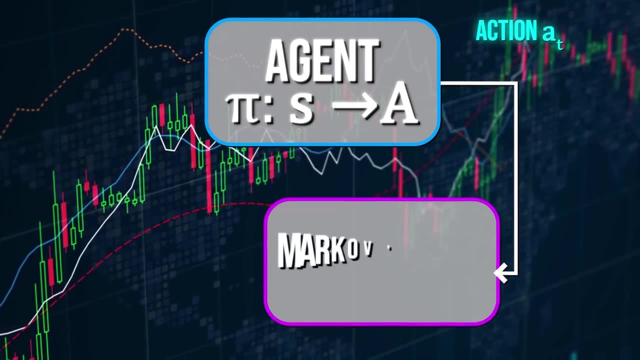 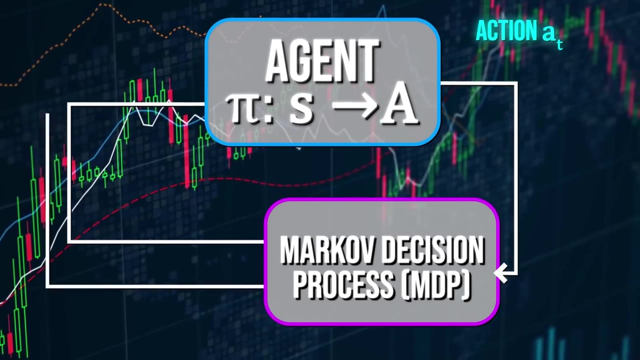 For any given stock, it can only perform three actions: buy, sell or hold. Buy: will buy as much stock as possible based on current stock prices and the amount of cash we have. while sell will sell all shares of a stock and add the generated cash to our cash balance. 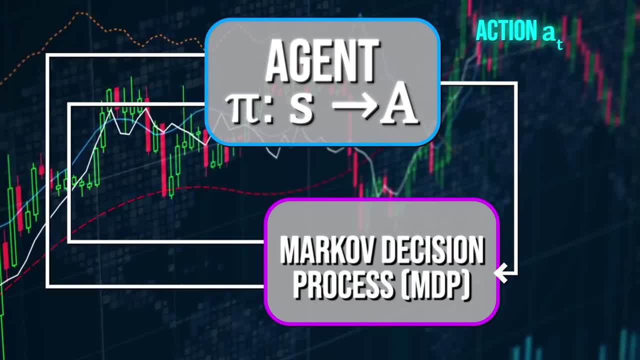 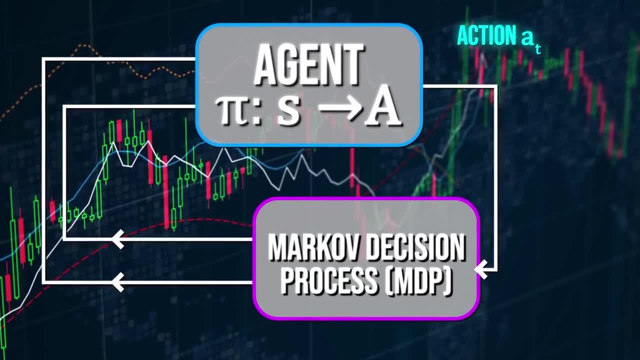 If we're buying multiple stocks, we would then equally distribute the cash we have for. each Hold, on the other hand, does nothing. So the number of actions at any given time step is 3 to the n, where n is the number of stocks in our portfolio. 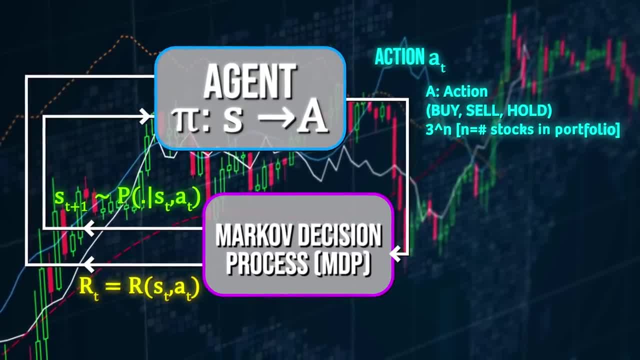 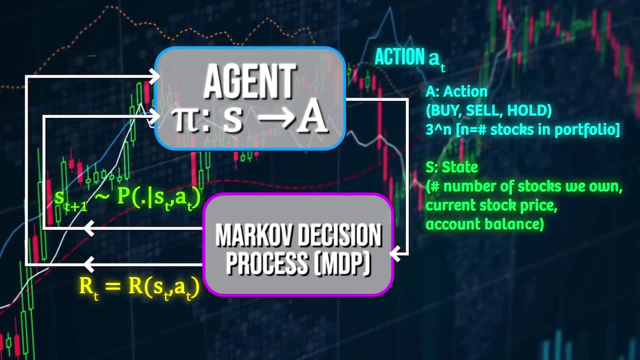 Now, at every time step, our agent will be in a state and from that state, will make an action For our state. in this case, let's consider it a combination of the current stock price, our account balance and the number of stocks we own. 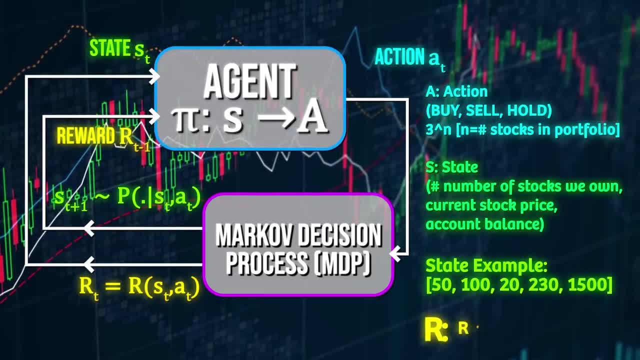 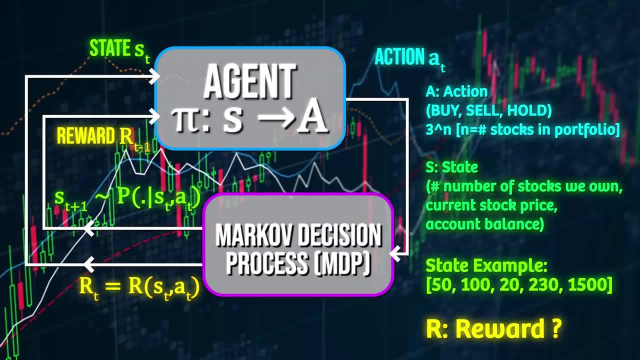 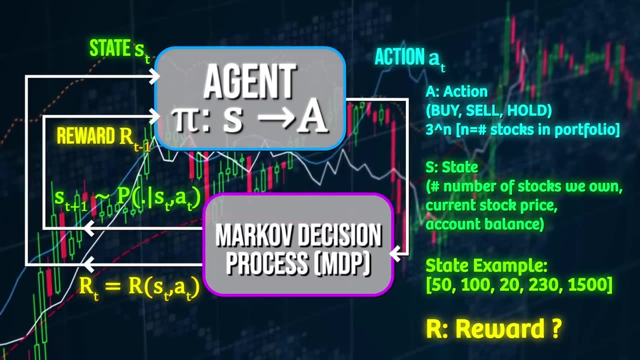 So, for example, if we own 50 shares of IBM, stock 100 shares of Microsoft and 20 shares of Qualcomm and have $1,500 in our balance, we can represent our state as an array which contains the amounts and prices of each stock, as well as the total account balances we have. 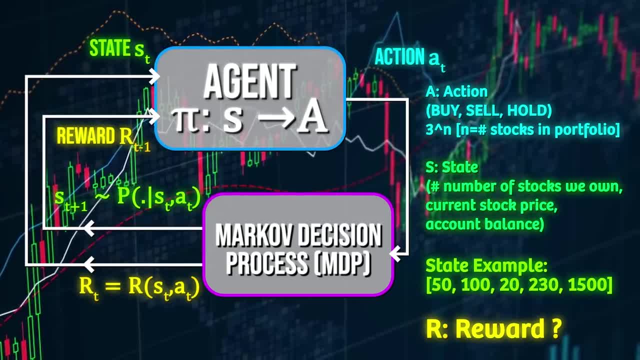 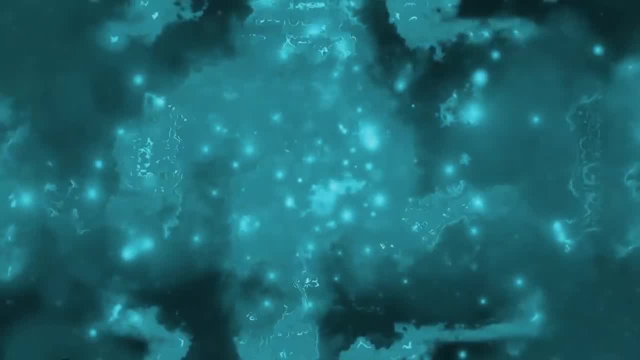 So it's this state category of the MDP that will contain any and all data that our algorithm could learn from, And we can add more to it later. but let's start simply. If we simply plot out the amount of capital we have for 3 time steps, we'll see that the 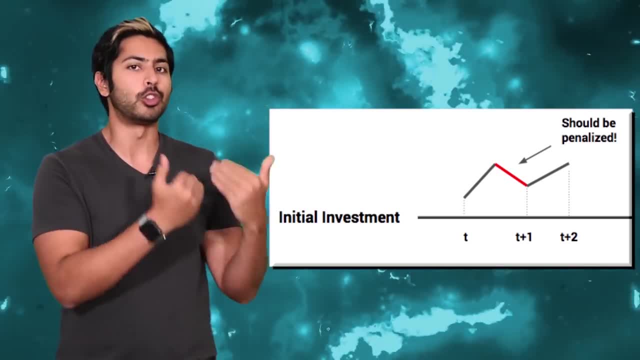 first two ideas for our reward won't help the agent learn from the difference in value between each time step. So if we simply plot out the amount of capital we have for 3 time steps, we'll see that the first two ideas for our reward won't help the agent learn from the difference in value between each time step. So if we simply plot out the amount of capital we have for 3 time steps, we'll see that the first two ideas for our reward won't help the agent learn from the difference in value between each time steps, So we'll go with the third. 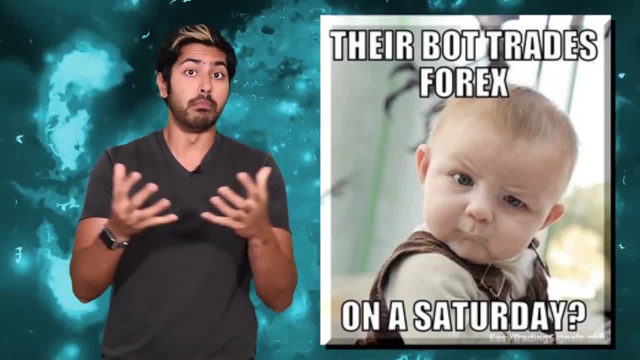 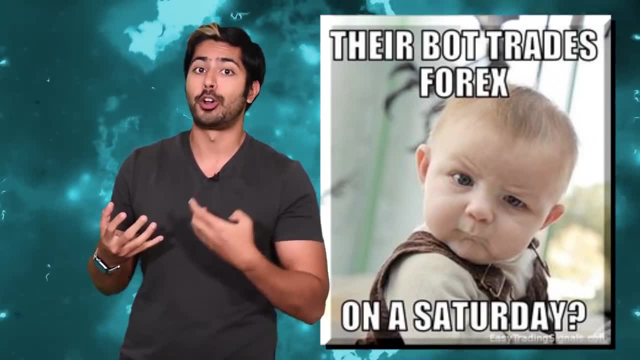 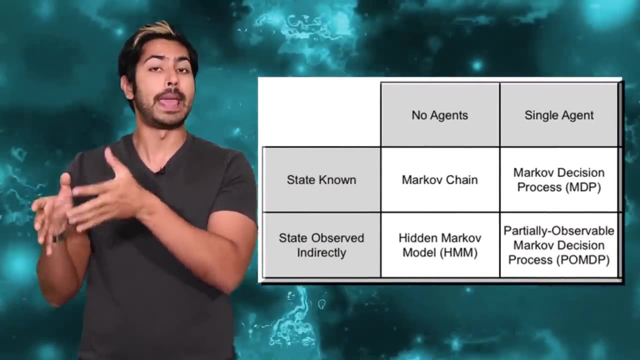 In this exchange environment we've defined, there are actually multiple agents, meaning there are other traders with their own respective account balances and open limit orders that are affecting prices. Unfortunately, we don't have access to their data, so we're dealing with a partially observable Markov decision process. And because it's partially observable, 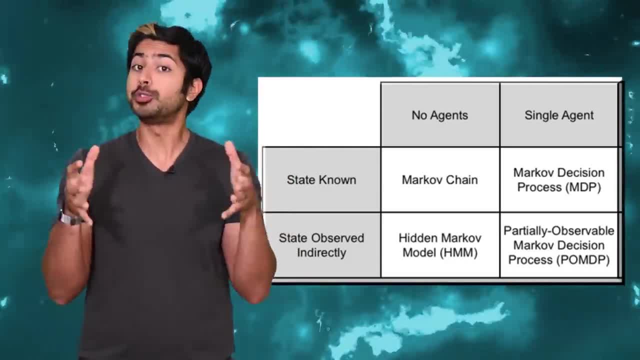 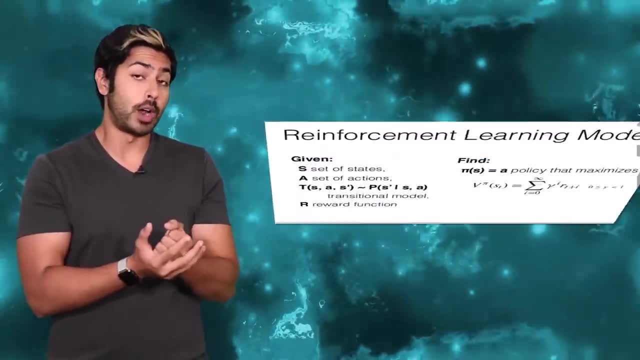 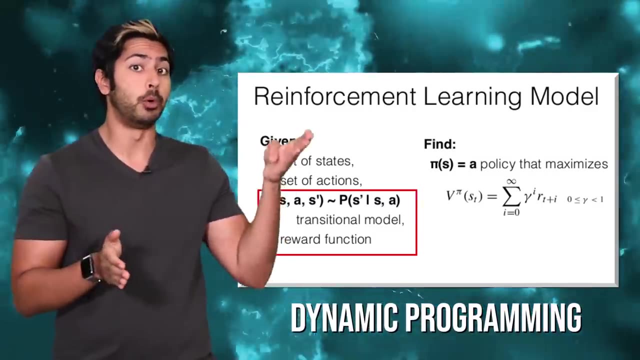 and we don't know what a full state looks like. we also don't know what either either the reward function or transition probability looks like. Dynamic programming is a technique that we'd use, if we knew these two terms beforehand, to compute the optimal policy. 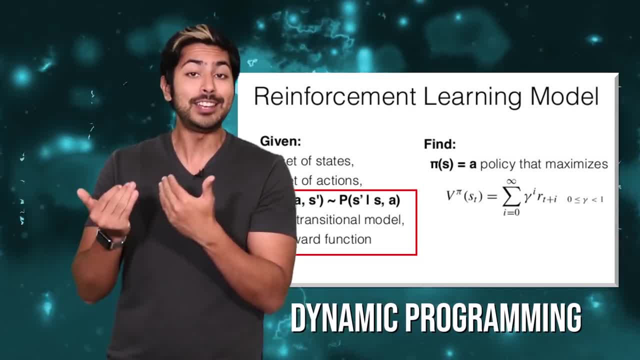 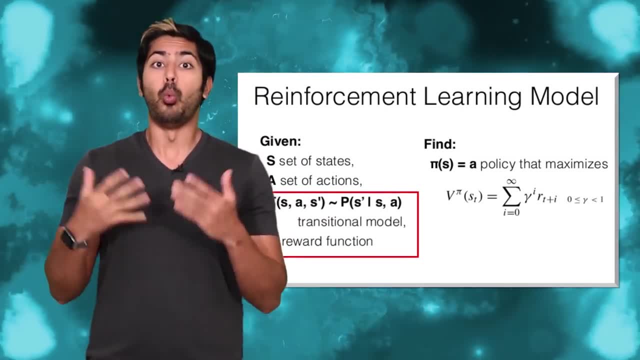 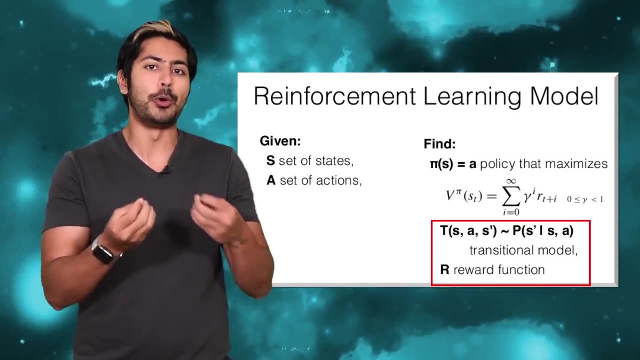 But since we don't know them beforehand, we could instead use another model-based reinforcement learning technique to learn these two functions. Once we do that, we'd be able to compute the optimal policy, because we'd eventually learn what the effect is going to be of taking a particular action. 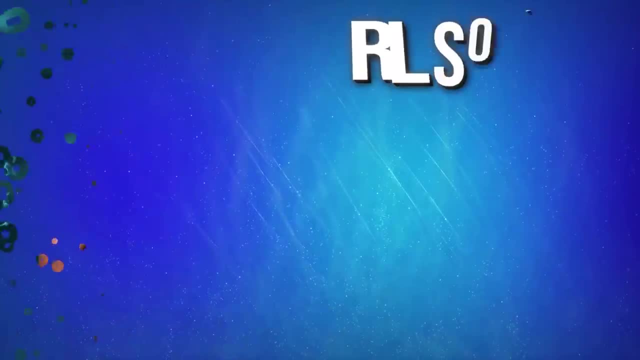 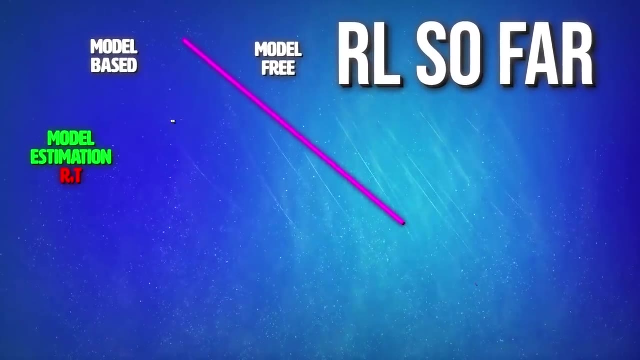 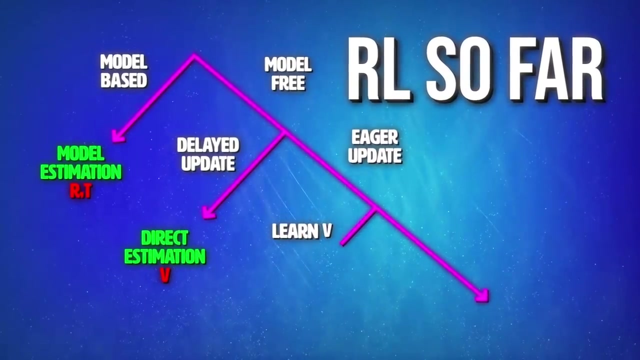 in a particular state. But what if we didn't need to explicitly learn these two functions? What if we could just learn the mapping from states to actions directly? We could compute a policy without needing to construct a full model of our environment, model-free reinforcement learning. 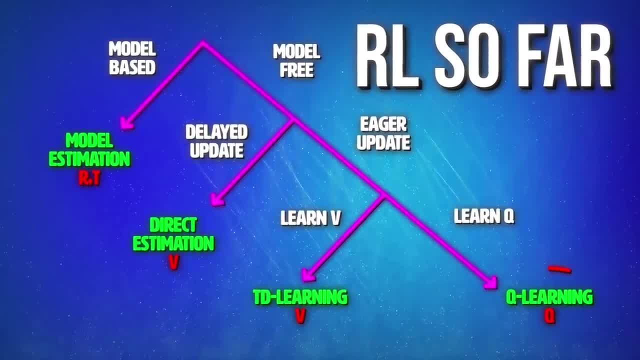 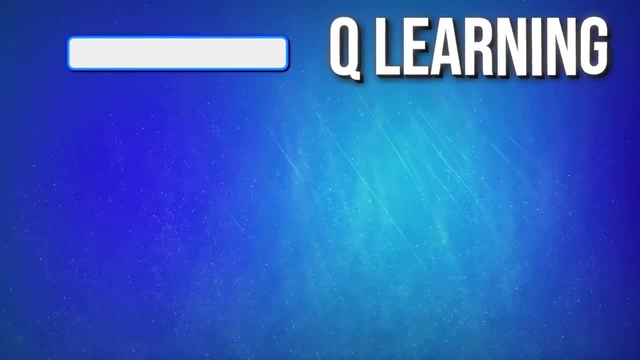 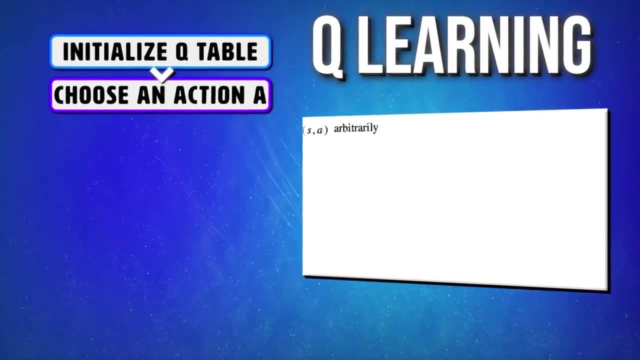 That'd be much more computationally efficient. so let's start with that. Of all the model-free techniques, Q-learning is the most popular. In Q-learning we define a function, denoted as Q, of S and A. This represents the maximum discounted future reward. 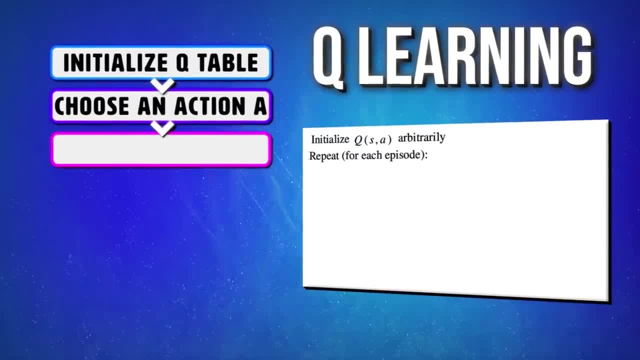 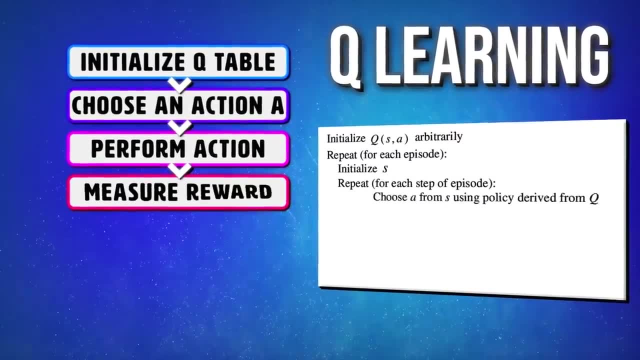 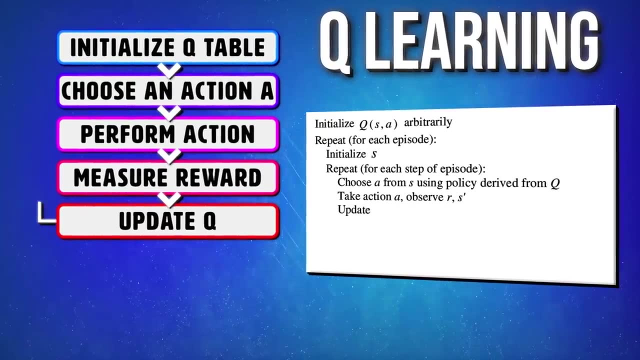 when we perform an action in state S and continue optimally from that point on. It's also called the action value function, since it measures the value of an action. We can think of this function as the highest possible account balance we can have at the end of a training episode. 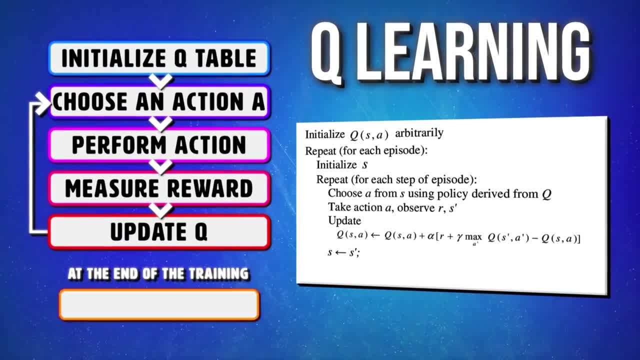 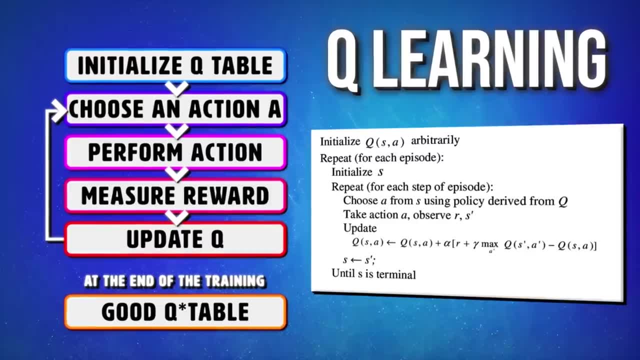 after performing action A in state S. It represents the quality of a certain action in a given state. In our case, our possible actions are either buy, sell or hold. Once we have this Q function, it will rate all three. Then we can just pick the action. 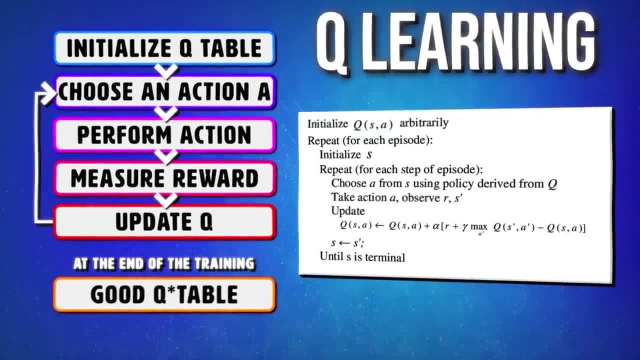 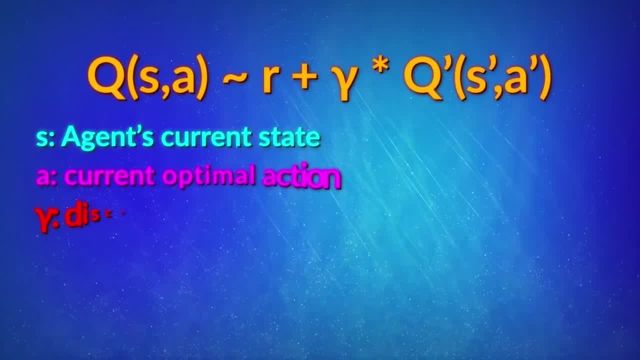 that has the highest Q value. So how do we compute this Q value? We can express the Q value of state S in action A in terms of the Q value of the next state. This is called the Bellman equation. It says that the maximum future reward 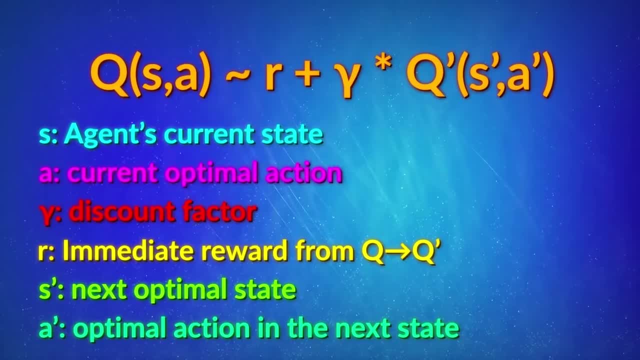 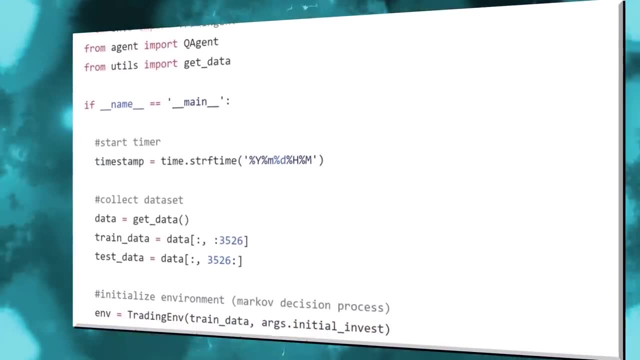 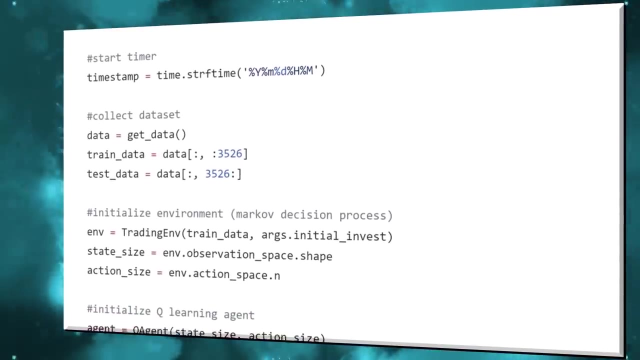 for this state and action is the immediate reward plus the maximum future reward for the next state. The great thing about the Bellman equation is that it lets us represent the value of a given state in terms of the value of the next state. It mathematically defines a relationship. 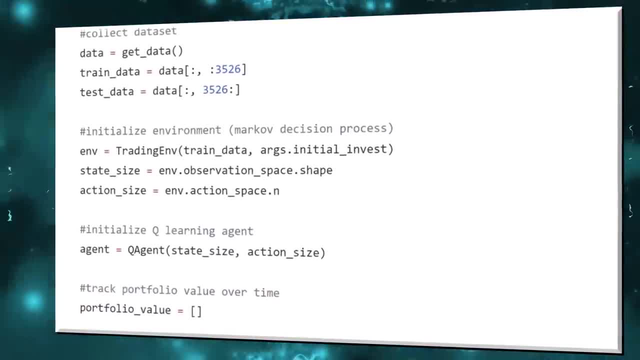 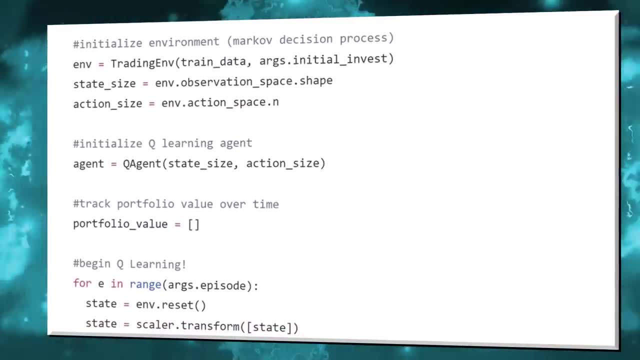 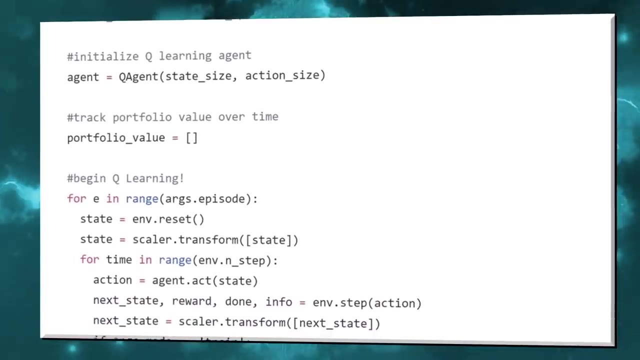 between states, which makes it possible for us to approximate the Q function. In the most simple case, the Q function is implemented as a table with states as rows and actions as columns. We'll initialize Q randomly, then observe the initial state S, which is going to be an array. 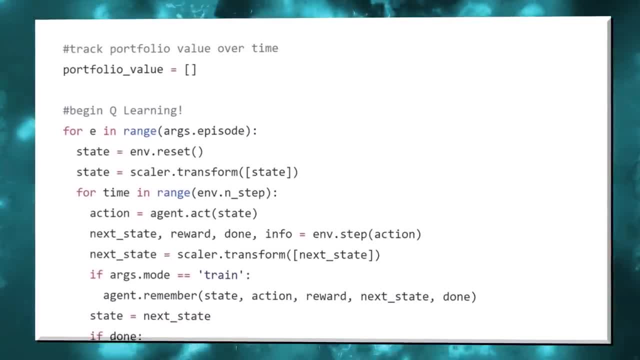 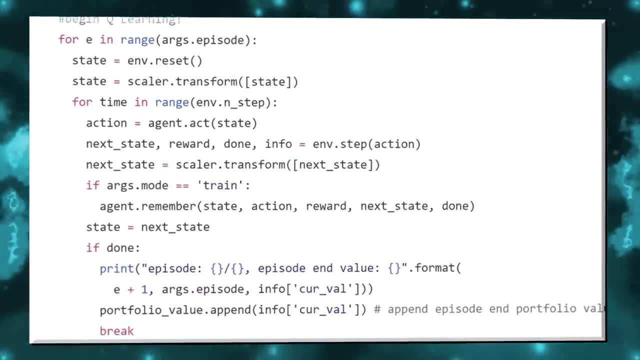 Then we iteratively compute the following four steps: We select and execute an action, then observe the reward and new state. Using these three values, we use the Bellman equation to update our Q function, then set the current state to the next state. 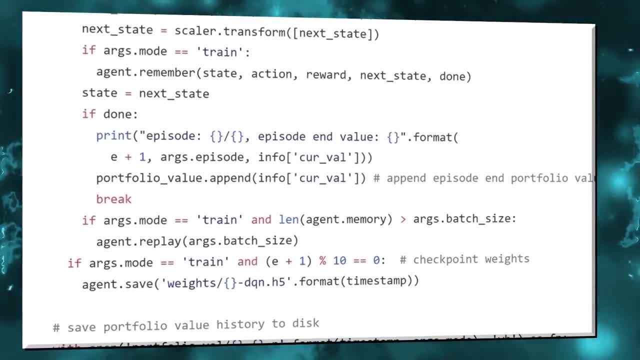 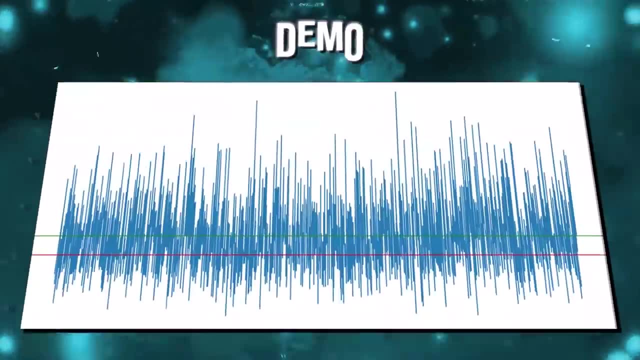 We just keep repeating that process for as long as we want to set an episode for, Based on just the data we have given our model, we can view the performance in this plot. The red line is our initial investment and the green line is the average after 2,000 runs.